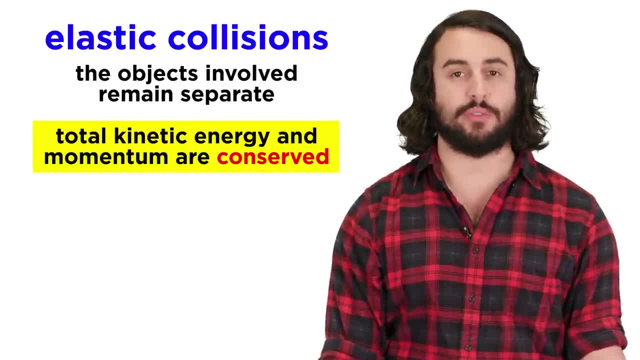 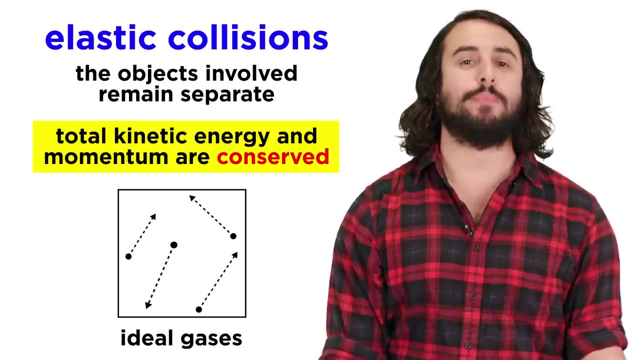 elastic collisions, total kinetic energy will be conserved, as well as the total momentum of the system, So the objects will bounce off of one another with no energy lost whatsoever as a result of the collision. We approximate collisions between atoms and molecules as being elastic. 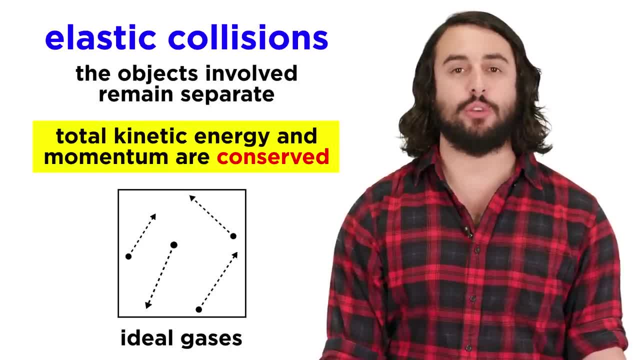 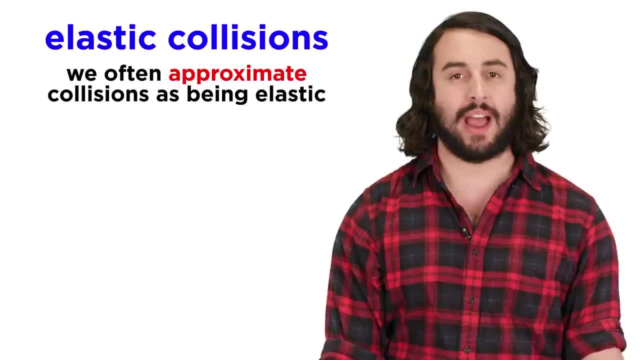 when we refer to an ideal gas, just the way we do with billiard balls. There are many other examples of collisions that aren't completely elastic, but we can treat them that way, like when a soccer player kicks a ball, since the player's foot and the ball do indeed remain. 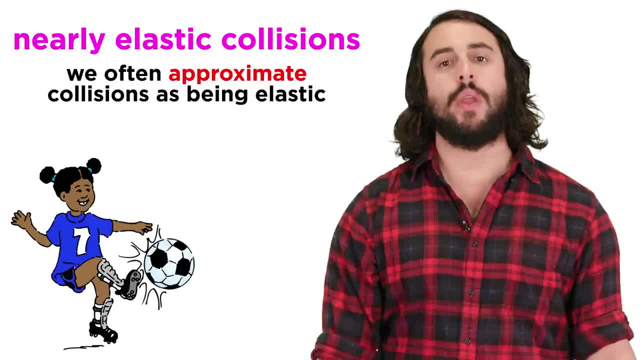 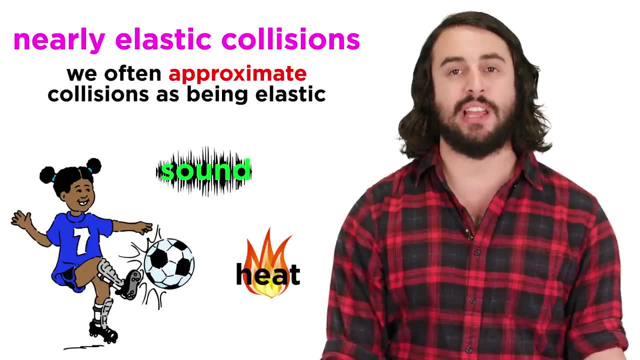 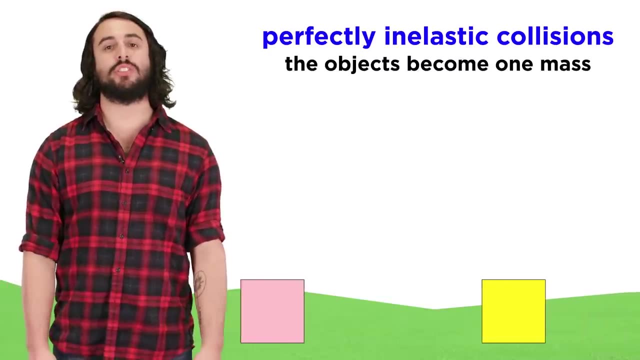 completely separate after the collision. We would refer to all of these scenarios as examples of nearly elastic collisions, since some kinetic energy is lost to heat and sound in each case. Perfectly inelastic collisions are those in which two separate objects collide, after which they move together as one mass. 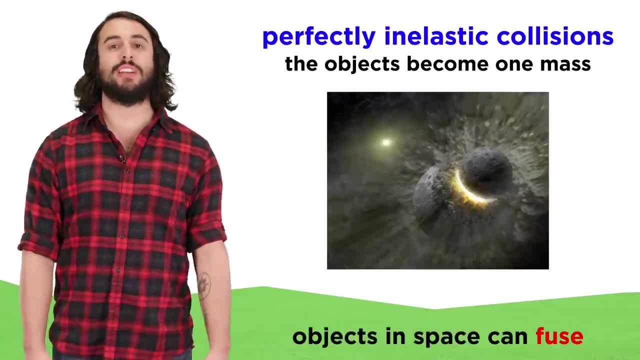 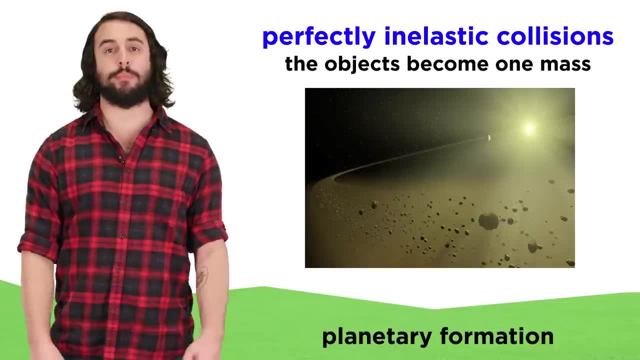 Sometimes, when celestial bodies collide like two asteroids, the collision is inelastic and they fuse together to form a larger body- body. In fact, this is how all planets begin to form, including the Earth, over the course of millions of such collisions. 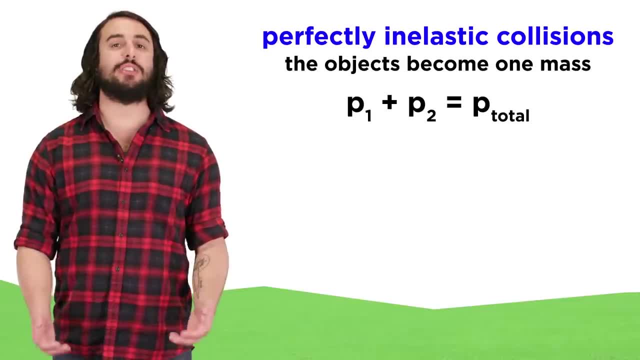 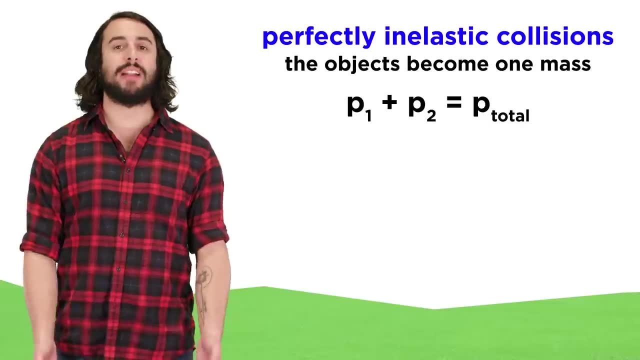 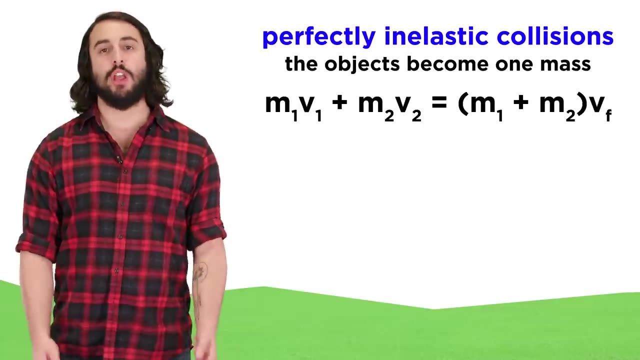 When we examine perfectly inelastic collisions, it is easy to analyze momentum, because we can treat the two objects as a single object after the collision, with a momentum equal to the sum of the two individual momenta. This is illustrated by the following expression: where m1 v1 plus m2 v2 is equal to the sum. 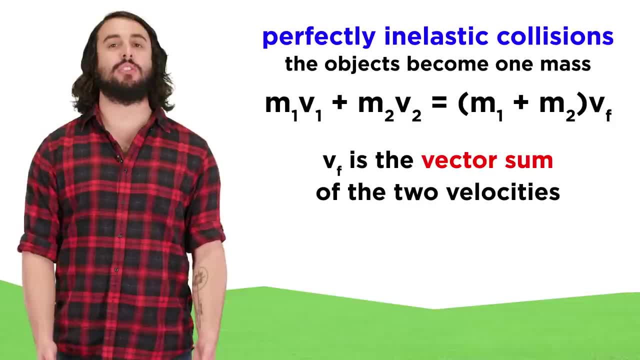 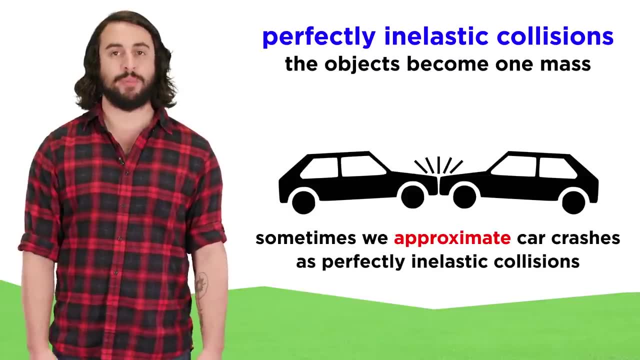 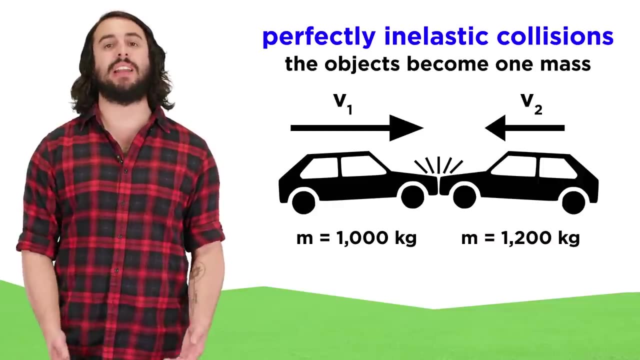 of the masses times v final, which will depend on the magnitudes and directions of the two initial velocities. This approach can also be used to model car collisions, whether the two cars were moving in the same direction or opposite directions. Adding the masses of the cars and combining the velocity vectors will tell us what will. 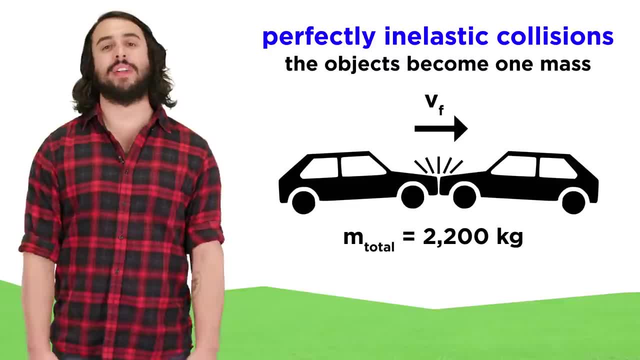 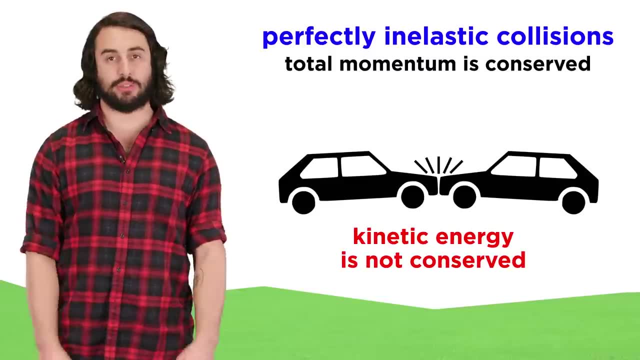 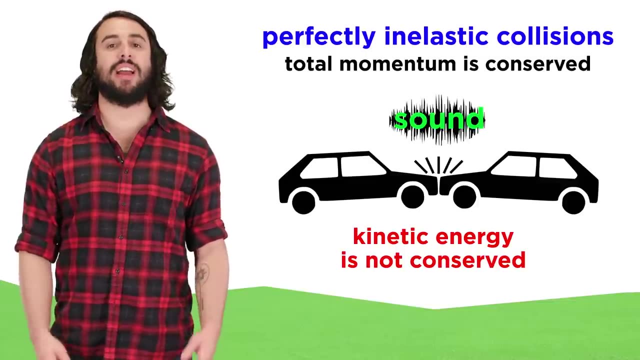 happen after the collision. We should note that during inelastic collisions like car crashes, total momentum is conserved, but total kinetic energy is not conserved. Much of the kinetic energy is converted into sound energy, which we hear as the sound of the crash, as well as heat energy and the internal energy of the new system which allows.